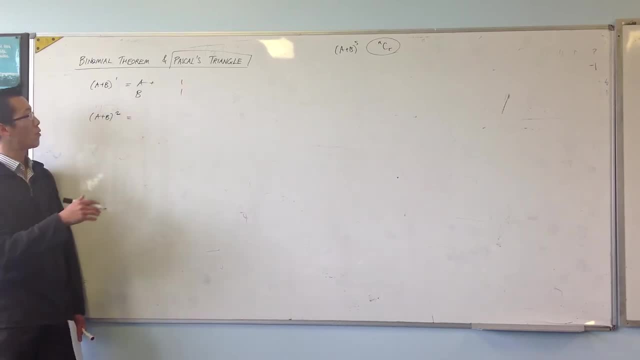 Now, what I know in advance, right, is that when I take these, I'm going to get a a's or a b's and b b's and so on, that kind of thing, right? So can I get from here? I want to build this expansion of these terms, okay. 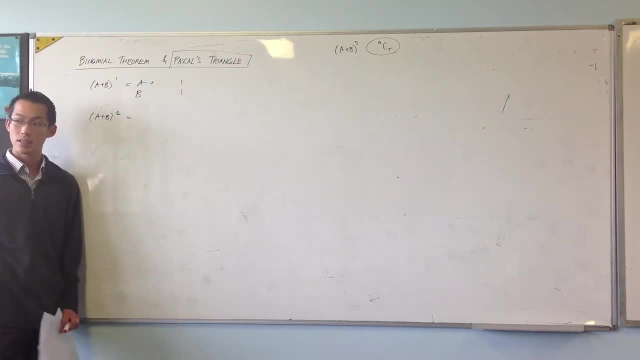 So, for instance, the first thing I would write down is: I'm going to collect like terms for a squared. a squared, So that's two a's in a row. Now, when I look at these two right, I can only build two a's in a row off this one right. 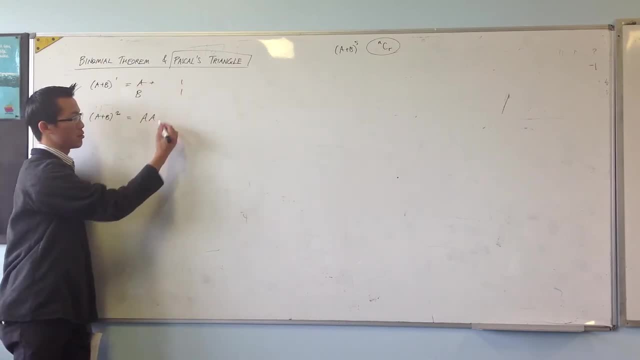 I'm going to take that one and add an a on the front. That'll give me two a's. okay, Now for my next row, my a b row. b a row. I want to get one of each letter, okay. 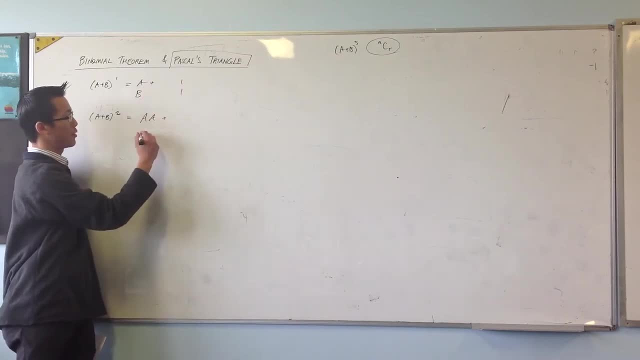 So you can see, I can build one off here by putting a b on the end, okay. And then I can build one off here by putting an a on the end, Okay. so these are my two terms, which have different letters, right? 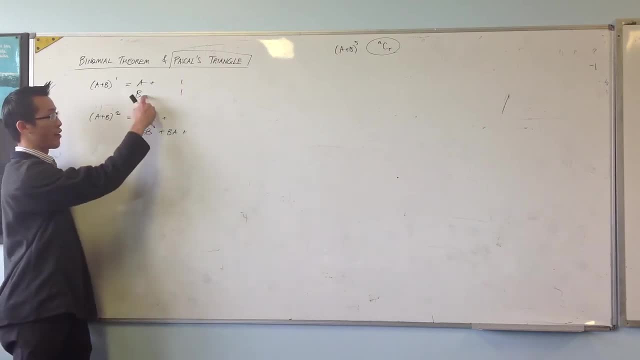 And then when I want to get my ones, which have two b's again, I can only build it off here. You can't get two b's if you start with an a. I'm going to start with a b and then add another one. 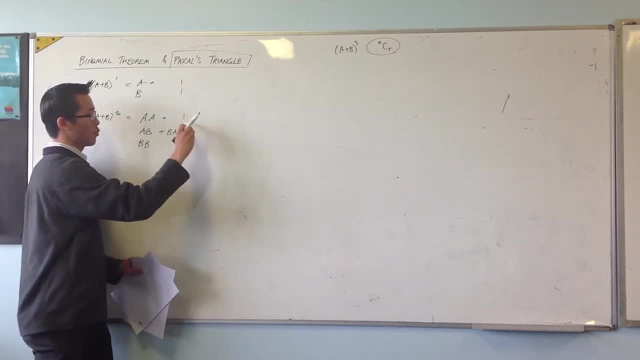 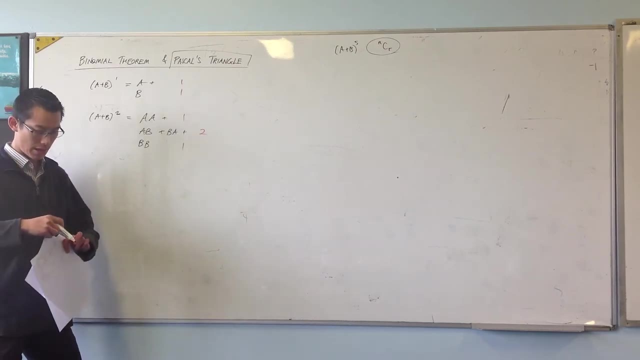 Okay, so can you see what I'm trying to do here? One that coefficient. we would normally have written this as two, a, b, Right, And then this one as one. okay, Now, the important thing to get is that: where did I get these two from? 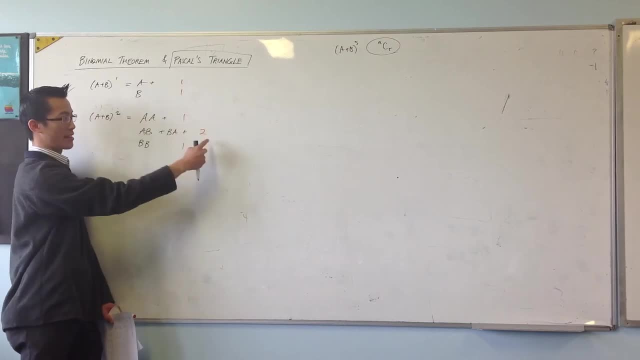 I've built them off each of these. I needed one from here and one from here, and that's how I got two. all right, Let's go again When you raise the power up one more time, okay, Well, the first thing I want to write down is: how many a cubed am I going to get right? 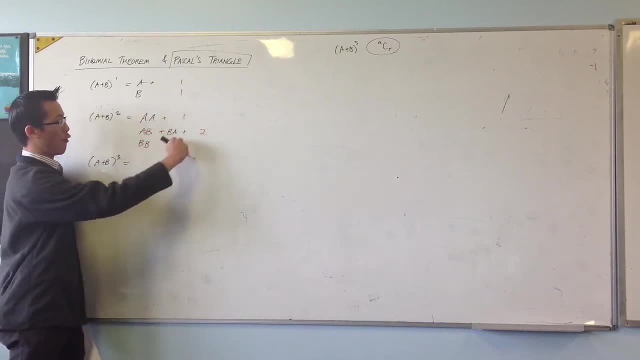 Well, if I want to build three a's, okay, you look at all four of these terms. which one can I use? Well, the only one I can get three a's off is this one, Right? So I take that and I add one more a, okay. 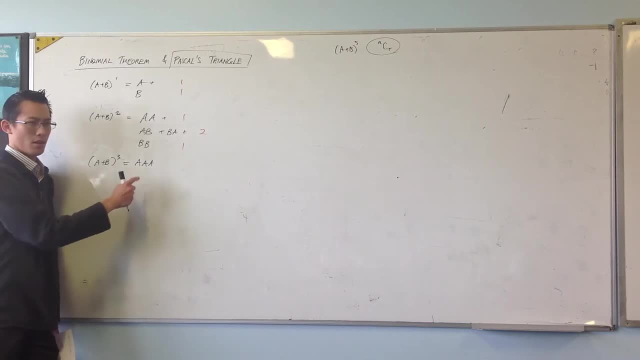 I can't get three a's out of any more of these terms. All right, my next one is a squared b, so I want two a's and one b. How many of those can I get? Well, you can see that I can get two a's and one b from any one of these terms, except this one. 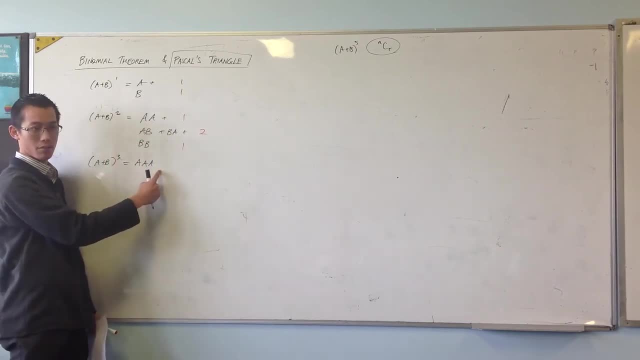 Can you see that Once I've got this, I can't get two a's in there because they're all going to have three terms. So I can go: this one, this one or this one I can build. let's see here. 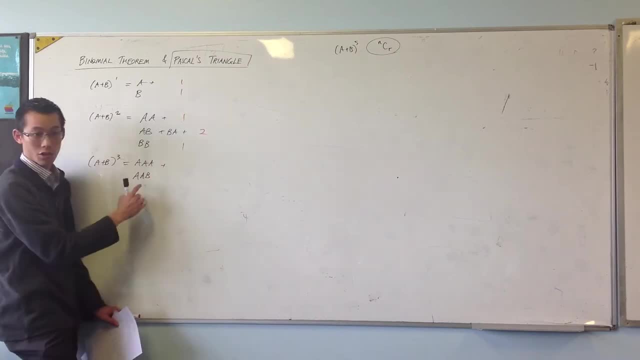 put a- b on the end of this one. So I've got two a's and one b. Put an a on the end of this one. You get a, b, a And then put an a on the end of this one as well. 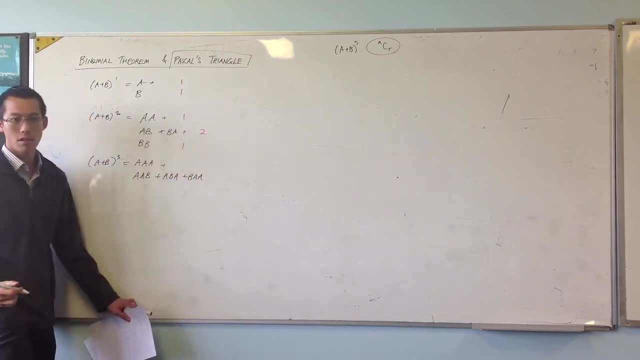 So I get b, a, a. So these are all the terms I could possibly build which have two a's and one b. Right, And I'm done. I got that, that row right. I got it by looking at all three of these terms. 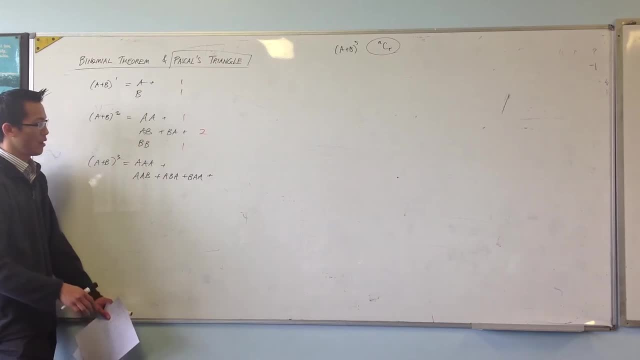 I had to take those two and then I add those two. Right, Alright. what about two b's and one a? How many possible ways can I build that? Well, I can build two b's and one a off of every term, except for that one. 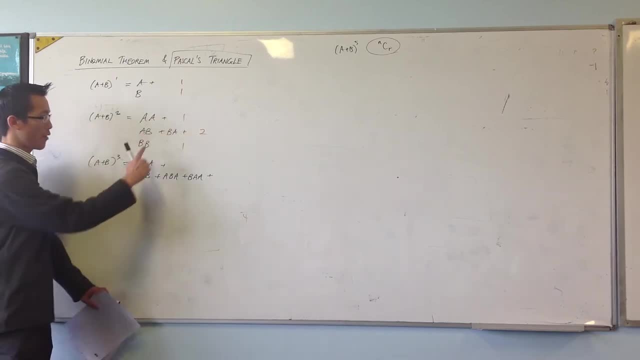 Because I can't fit two b's in there, because then I'm going to have four letters. So if I go these three here I want two b's and one a. So if I take this one and add a b on the end, 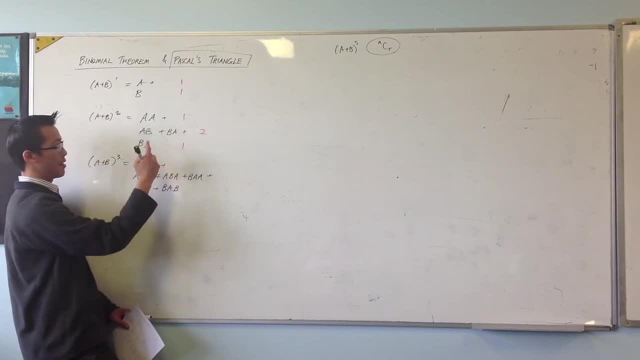 Take this one and add a b on the end, And then take this one, And then I want to add a b on the end because that will make it three b's Right. So I'll add an a on the end, Okay. 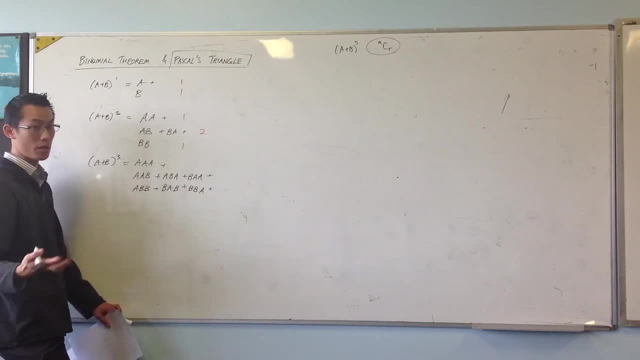 So here are my three terms: Two b's and one a. So normally I would write a b squared. And then, lastly, of course, I've got my three b's, And there's only one way. only one of these can lead me into a triple b. 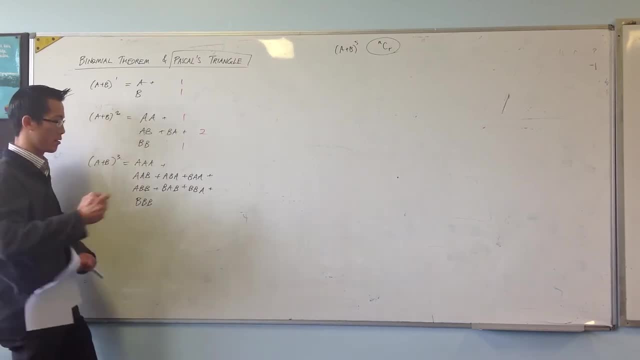 Right. So can you see, right? I'm going to try and draw some arrows here to draw the connections. I've got one term here, three terms here, three and one Right. Where did these three terms come from? It came from taking these two rows and every term in them and modifying them in some way. 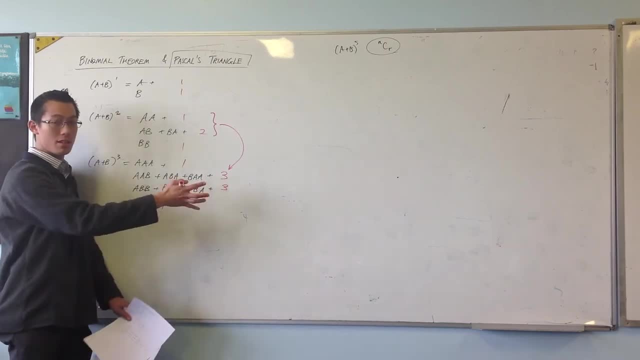 Right, So that's how I got three. I got this three. in a similar way, I took these two rows here, Right, Okay, Let's do it one more time and then hopefully that will be enough and you'll probably run out of space anyway. 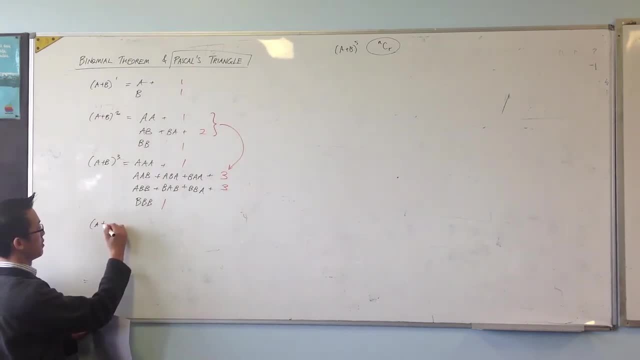 Let's raise it to the power of four. Okay, All right, Now can you see the way I'm building this? If I raise it to the power of four, All of these words, as it were, that I'm going to get, at the end, they're all going to be four characters. 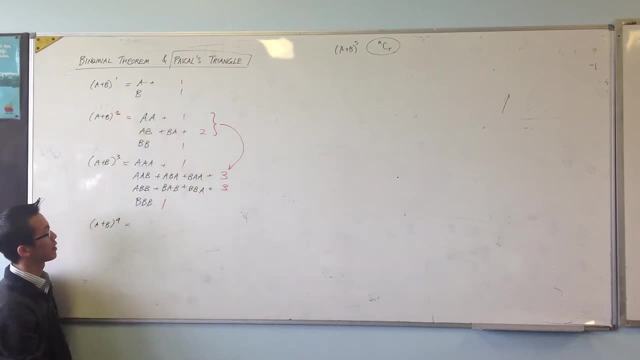 Just like these are all three characters, two characters, one character. Okay, So I want to make one with four a's. Well, out of all of these, there's only one I can possibly use, namely this one, Right. 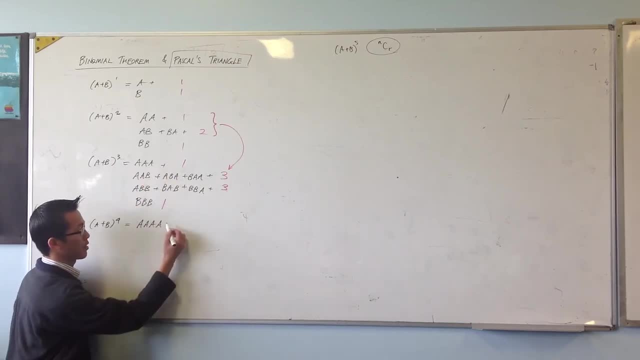 So that's why I'm just going to have one of him. Okay, Now I want. how many can I build where I've got three a's and one b? Well, can you see which ones I'm going to use? 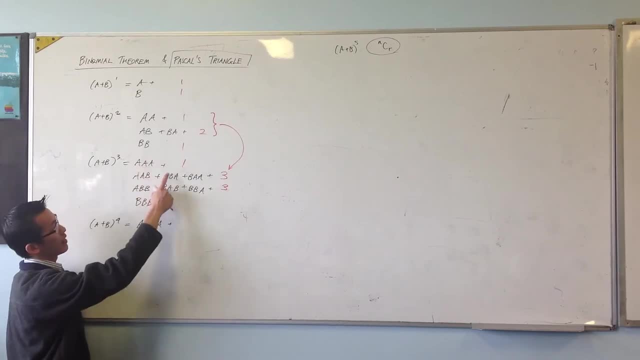 Right, I can get three a's and one b out of that. and I can get three a's and one b out of all of these terms, Okay, So here, how do I get that? I'll add a b on the end. 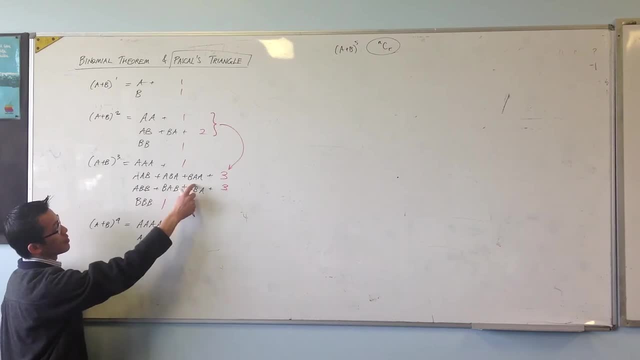 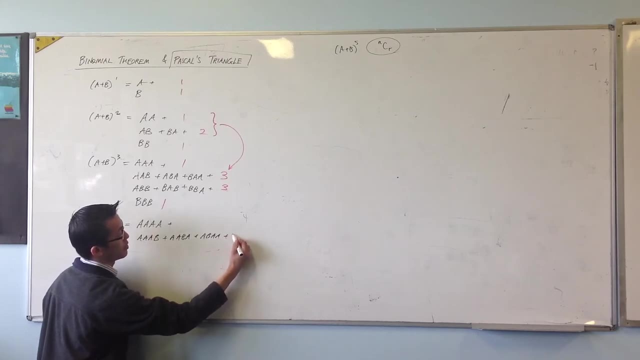 Right, And then for these ones I'm going to add an a on the end. I'll get a a, b a, a, b a a and b a, b a, And that's all I can do. 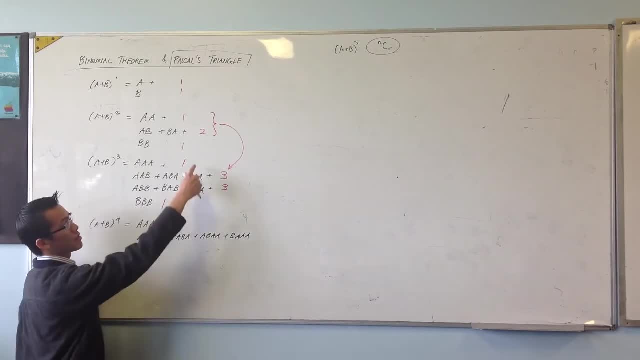 There's no other way I can get three a's and a b Right, So I use these two rows to build up this one, Right, And you can repeat the same exercise. for how can I get? oh, sorry, no. 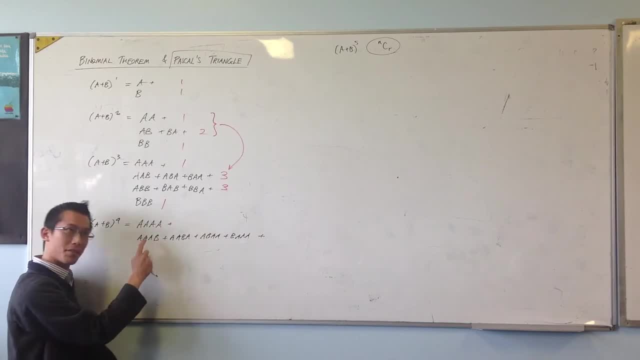 See, this is where I get a new row. So now I've got three a's and a b. Now I want to think about how many ways can I get two a's and two b's. Two a's and two b's. 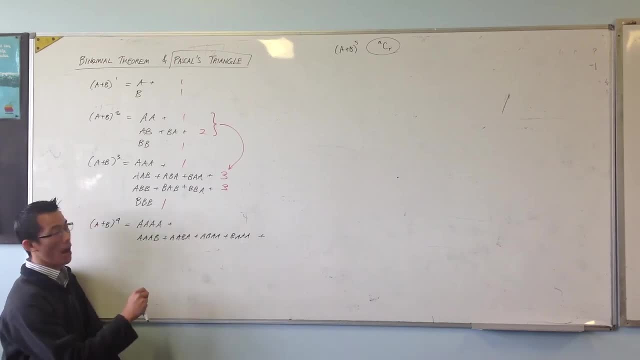 Now have a look at these two rows up here. Right, I cannot get two a's and two b's out of here. Right, Because I've already got three a's. Can't get two a's and two b's out of here, because I've already got three b's. 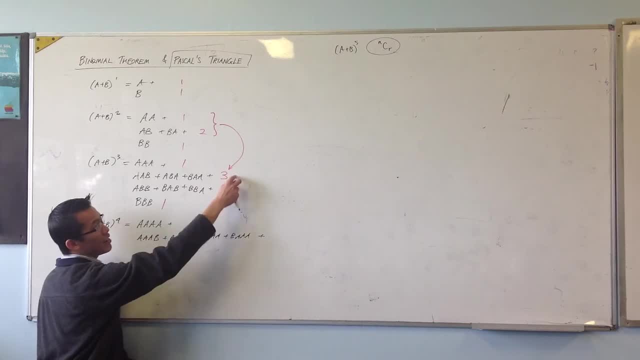 Right, But I can get two a's and two b's off any of these six, Right? You just have to add a different letter each time. So in this case, right, what would I add on the end? I guess I would add a b on the end. 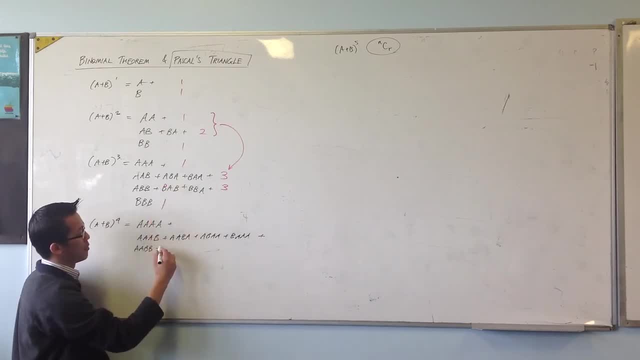 That'll give me two a's and two b's Here. I'll add a b on the end again, And then this one, I'll add a b on the end. Okay, So I've got two a's and two b's off all of these. 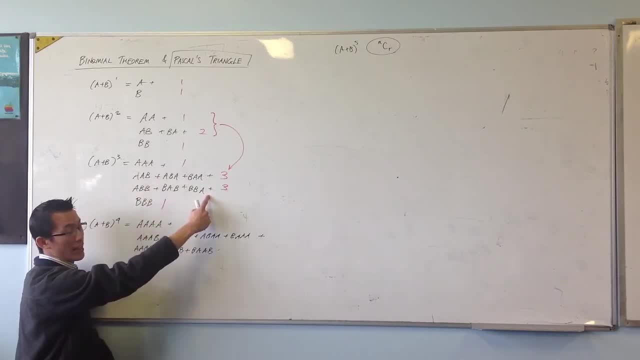 And here off this next row. how do I get two a's and two b's off here? Well, I get two a's and two b's, So I guess I'll add a on the end of every single term, Right? 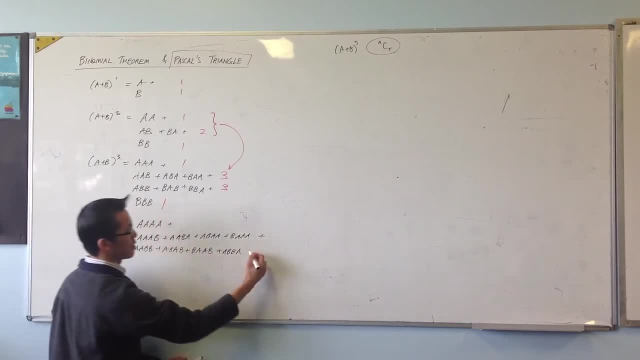 So this is going to be a popular European band. one of my favourite elephant cartoons from the past, almost, and whatever. that is Okay, So I added b onto the end of all of them. Okay, So you can see that. 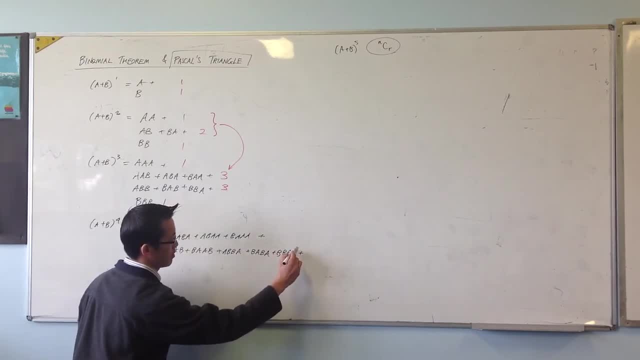 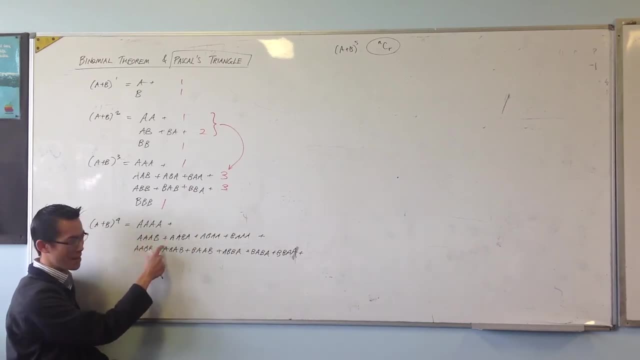 Yeah Sorry, Did I miss one A? Oh yeah Sorry, Thanks. a's and b's. They all look alike. I should have picked different letters, So three a's and a b, Two a's, two b's. 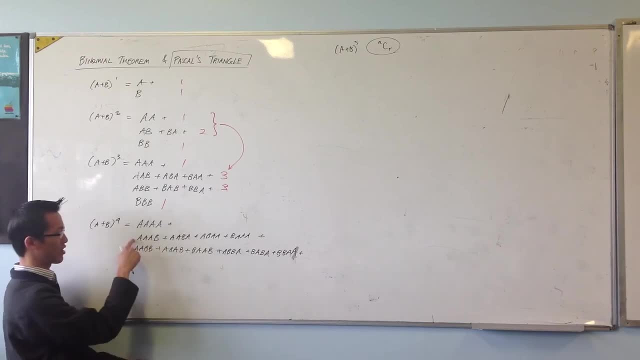 The next one is going to be three b's and an a, So you can actually just take this one and swap all the b's with a's. Okay, Three a's and a b, and then this one, of course, at the end will be four b's. 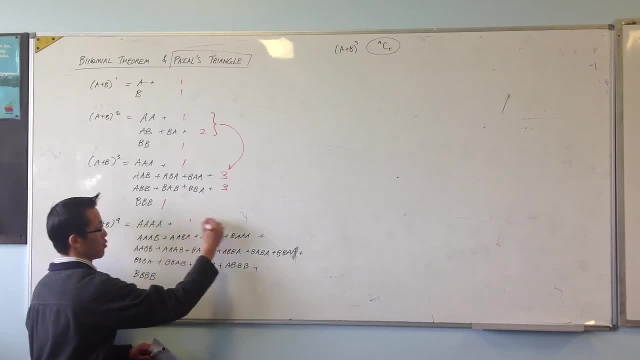 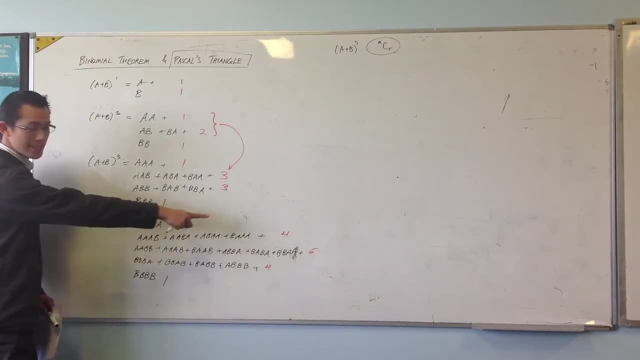 Right Now, when you do your count- okay, you've got your one, four, six, four, one- And the key to understand is: well, where did those numbers come from? Like, where did that six come from? 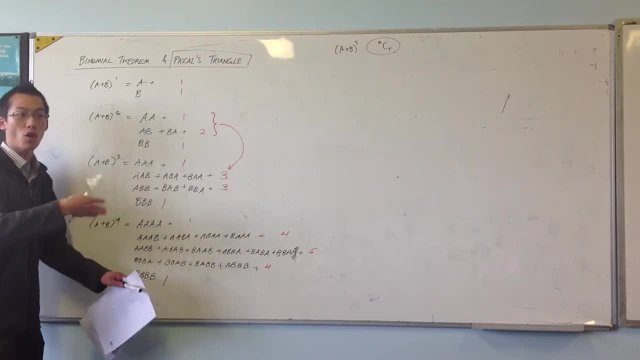 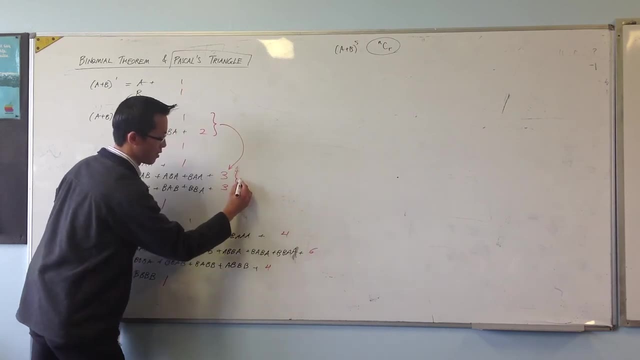 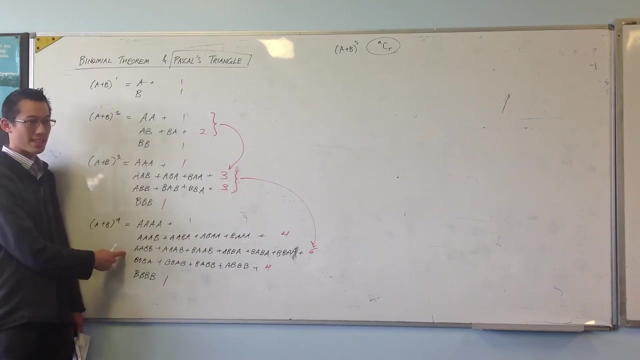 The six came from the fact that every one of these terms is built off of these two rows Right. Oh, that's a terrible brace. Let's try that again. That's better. Okay, These three and these three right turn into this six. 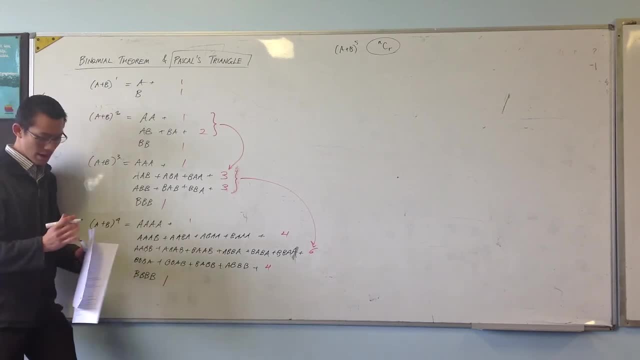 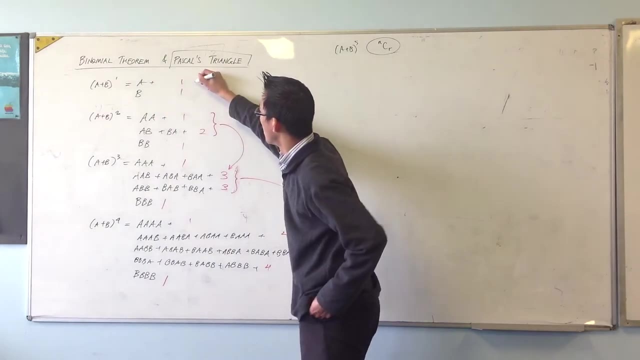 Okay, So can you see why. Now let's write down the actual coefficients. How would we normally write this expansion? We would ordinarily write a plus b, That's no problem. Here we'd write a squared plus two: a, b plus b squared. 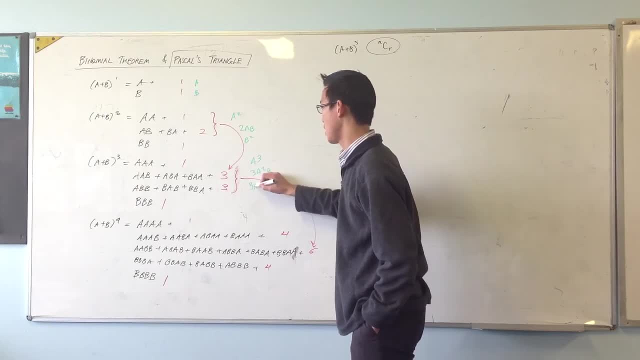 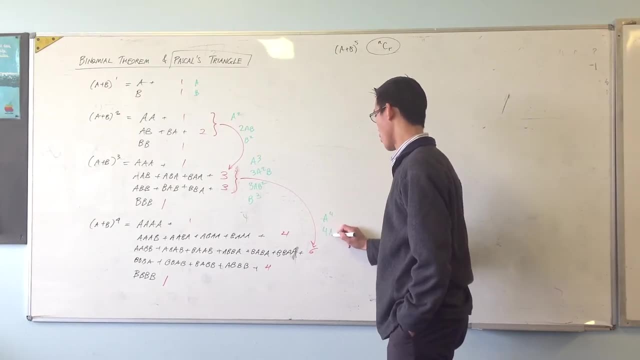 Here we'd write a cubed plus three a squared, b plus three a, b squared plus b cubed, And one more for good measure: A to the fourth, four: a cubed, b, six: a squared, b squared, A b cubed, and b to the fourth. 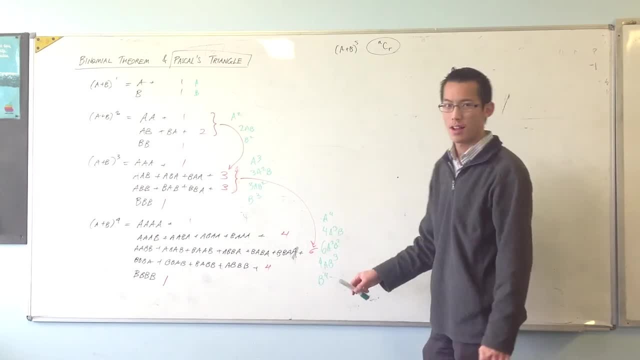 Okay, So you can see these coefficients here. they line up with Pascal's triangle, because solving this problem is the same as the way we build Pascal's triangle, Right, Which is you do. oh, I add these two numbers and you get three. 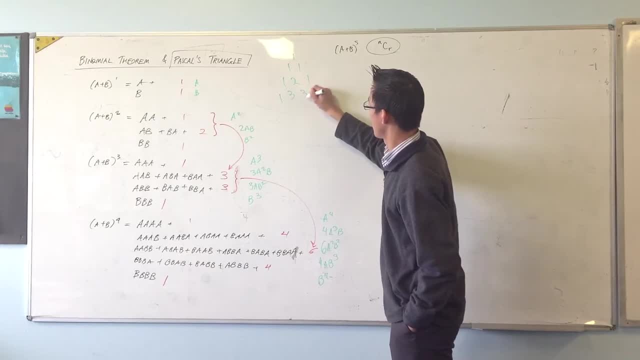 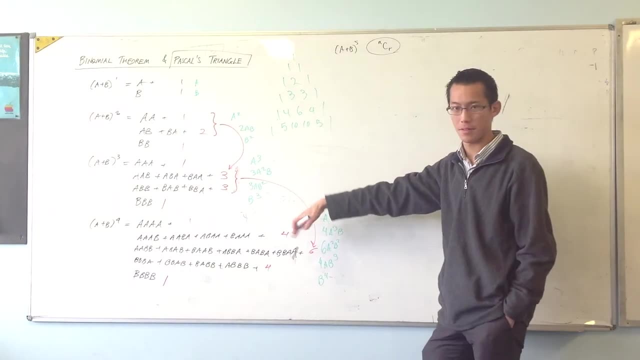 Right. So when you've got this kind of structure, even though you think of them as well, this one I just get from straight. you know, addition, Right, And this comes from algebra. Well, the algebra comes from the same rules of addition. 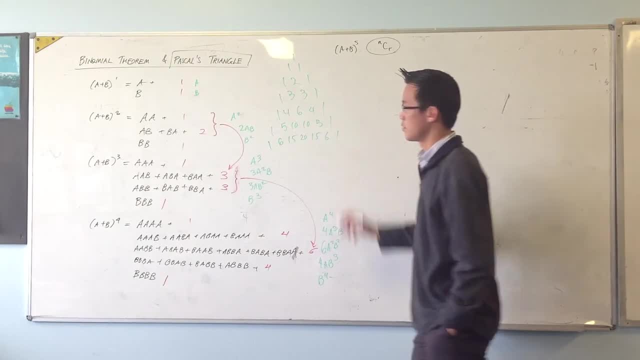 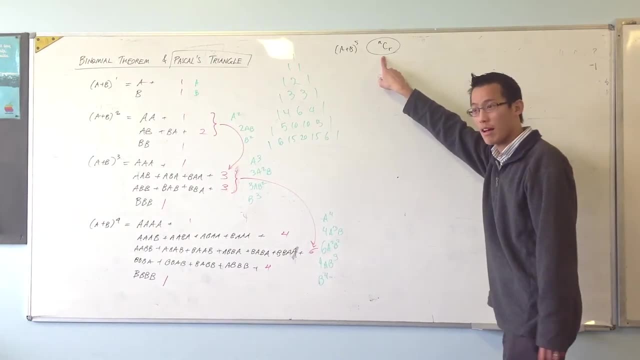 Right. Fifteen, twenty, sixteen, fifteen, sixteen, Alright. Now, remember, I said that this expansion idea right. I connected it to this Right. So now I'm connecting the expansion idea to this Right. Pascal's triangle. 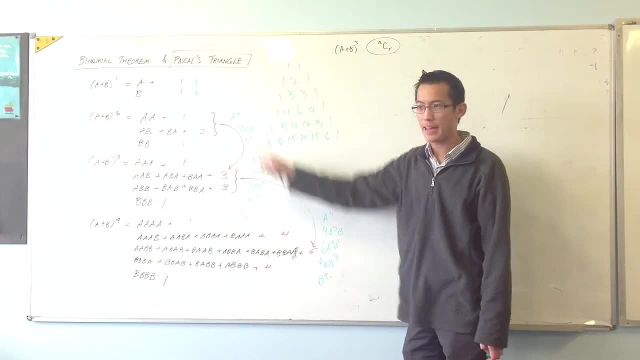 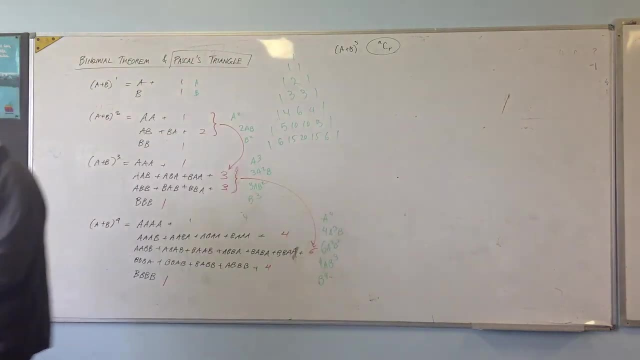 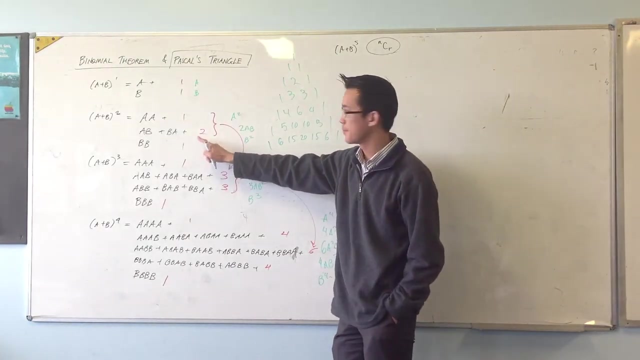 So, therefore, I can rewrite Pascal's triangle just in terms of NCR notation. Okay, So how does it work? Think about, say, this expansion here. Okay Now, what did we learn about binomial theorem? I asked you to write it in general form. 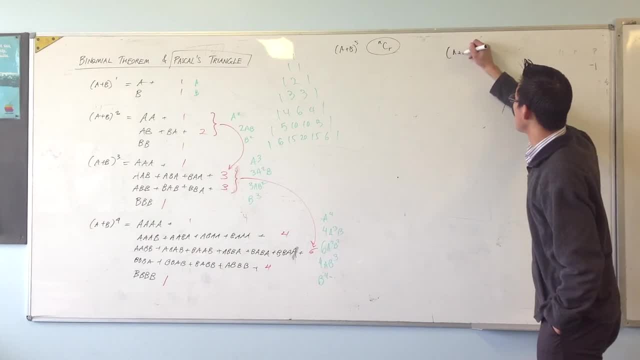 Do you remember? Have you got it there Where you've got like A plus B to the power of N? Okay, And your coefficients in all your different terms? Okay, What's the first coefficient, Do you remember? Choose zero. 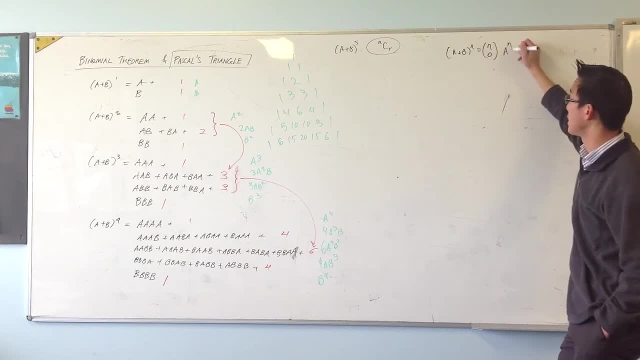 That's right. N choose zero- Okay. So you've got just A to the N And you do have no lots of B. And then the next one will be: N choose one- Okay. And then you've got one less lot of A and one more lot of B, and so on. 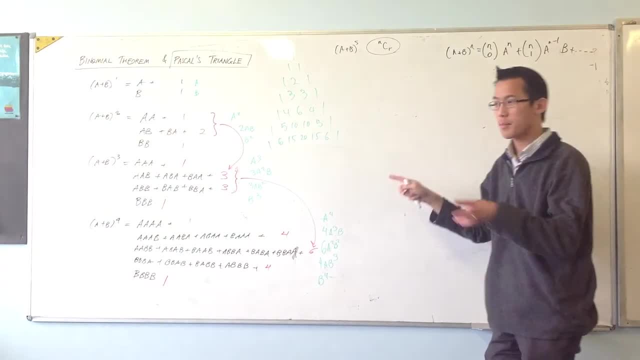 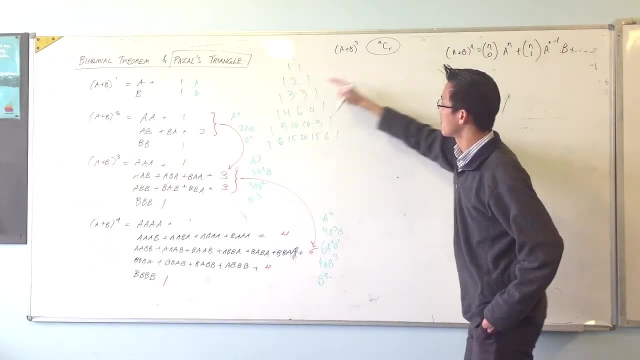 Right, Okay. So how can we use that here? Well, think about, say, this: row here: One, two, one, Okay. Where it came from? was this expansion? So it's going to be that one is really two, choose not. 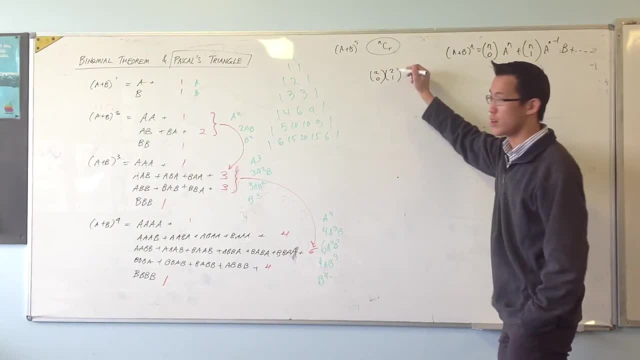 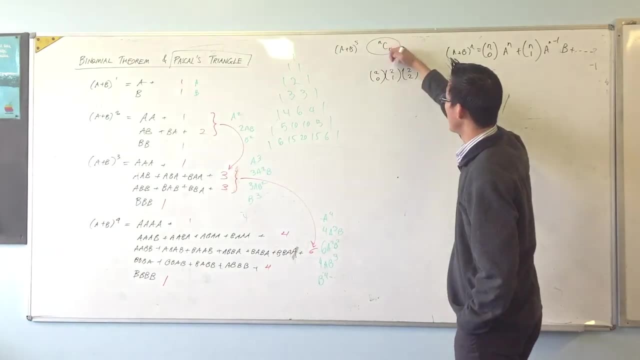 Right, This two is really two choose one And then two choose two Along the N. Okay, It just says one row, So I can write the whole lot in the same way. These are all twos, Right? The next row up will be one choose not and one choose one. 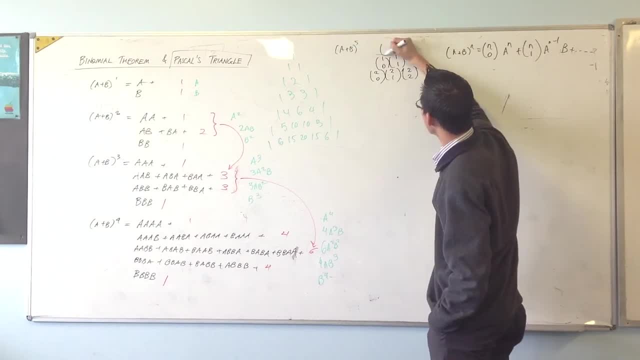 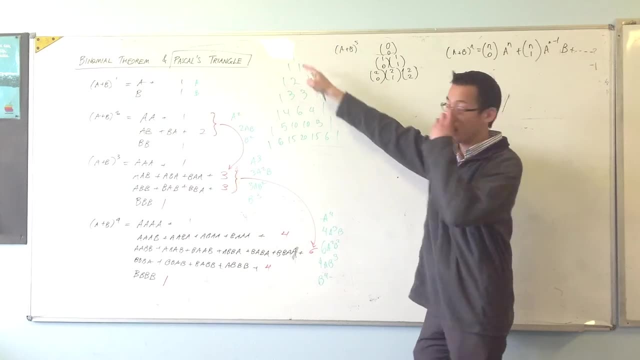 Okay, At the top, you've got not, choose not. You know, I've got no things and I want to choose none of them. There's only one way, Right, And every other row can also be built using NCI notation in exactly the same way. 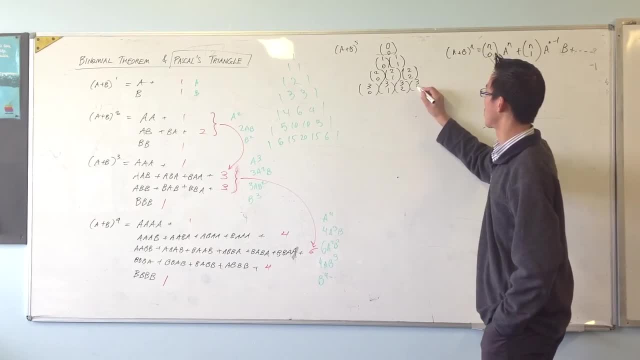 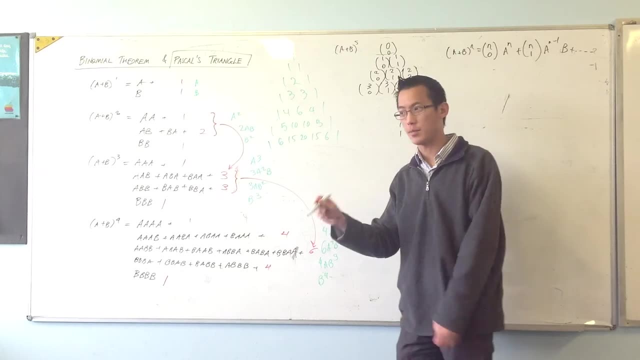 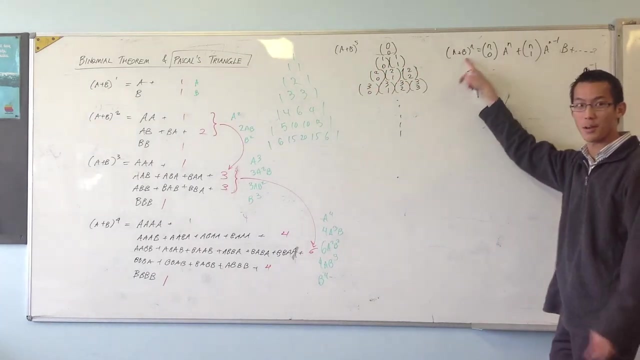 Three, one, three, two, three, three, Okay, And so on, Right, So this is a really important part. It's identified explicitly in the program, But you've got to get how this and these and this all connect to each other. 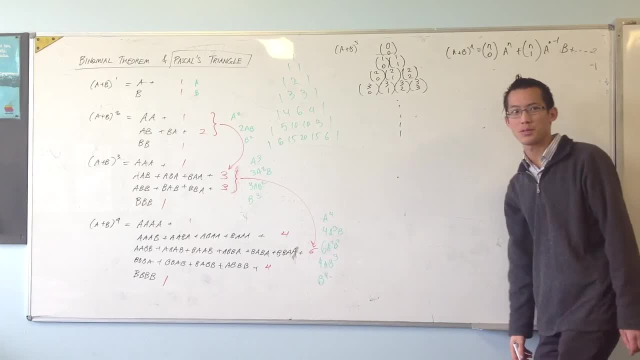 Okay, They're kind of like I was going to say two sides of the same coin, but it's three sides So and you can't make it geometric. Well, actually, a coin kind of has it's like the, it's the rim of the coin. 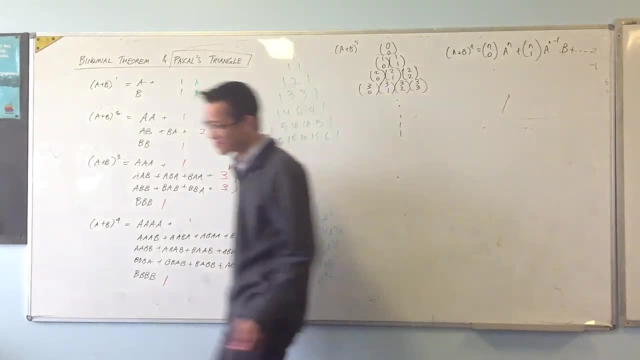 If it was a thick coin Anyway. 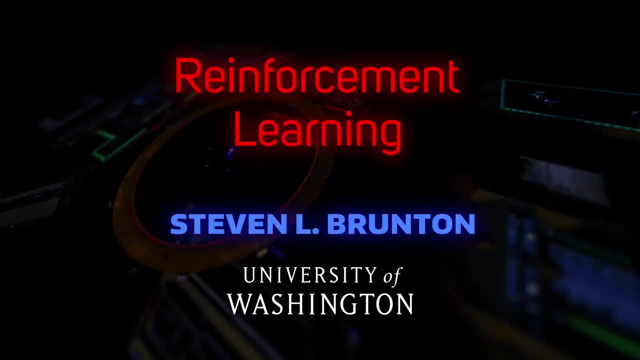 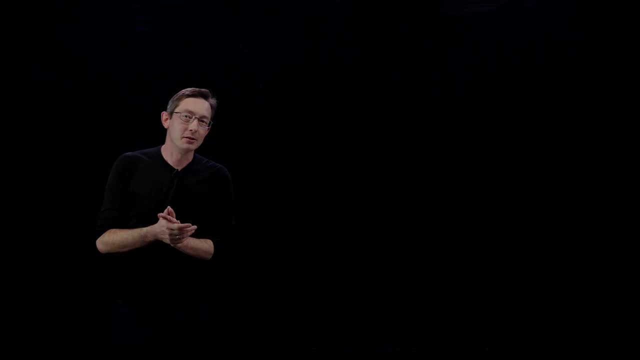 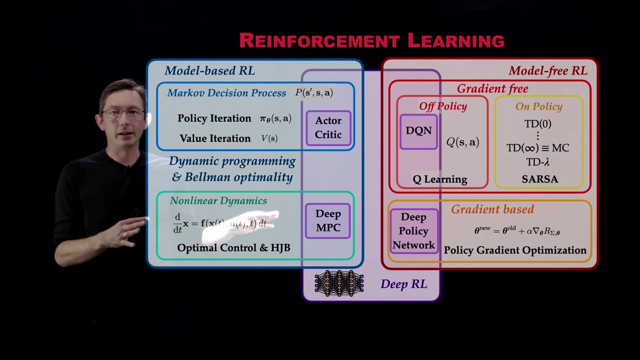 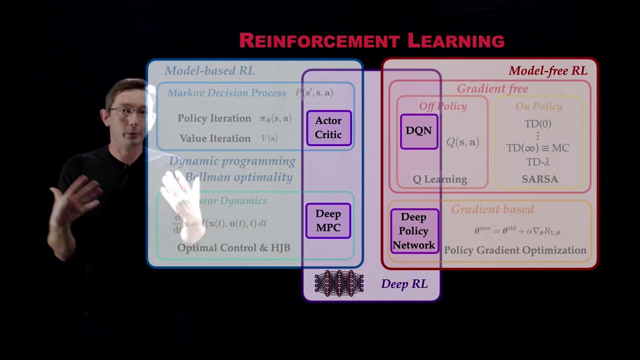 Welcome back everyone. So I'm really excited to continue this lecture series on reinforcement learning, And in this one I'm going to zoom in specifically on deep RL- deep reinforcement learning, or, said another way, reinforcement learning using deep neural networks. Okay, 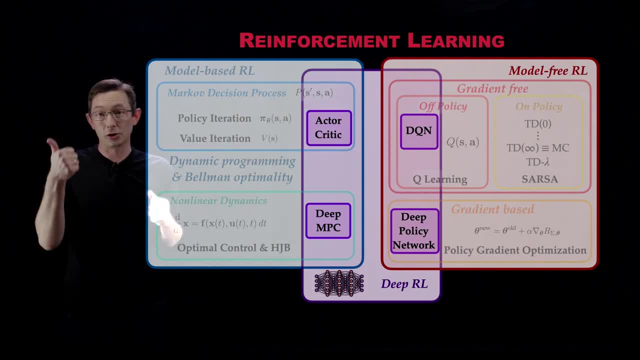 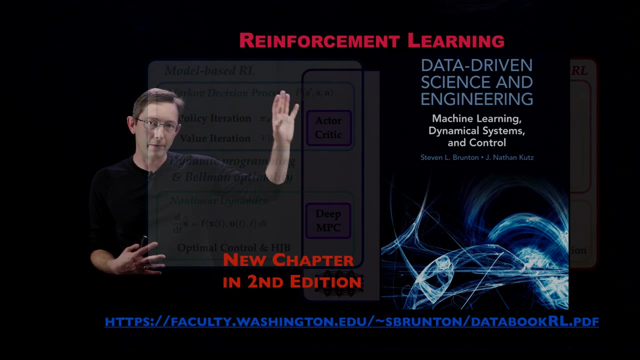 this is one of the most exciting trends both in control theory and in machine learning over the past decade, And there's just a ton of new and exciting results out every month, it seems. on deep reinforcement learning, Just a reminder: this is following roughly a new chapter.